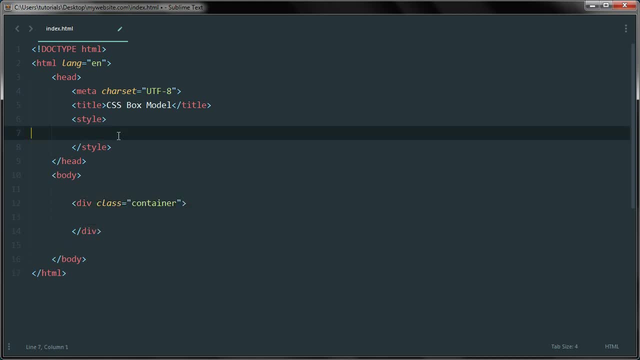 and this container will be a thousand pixels in width. So let's do the container here And we will apply a width of 1000 pixels. We will do a height of 500 pixels. I'll add a border to this, just so it's much easier to see. I'll do a one pixel solid red border And we will center. 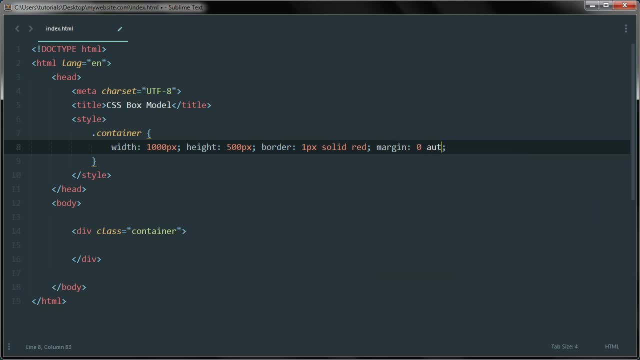 align this by using margin zero auto. So nothing new. We can see that in the browser. this gives us a center aligned border. So let's go ahead and do that. So let's go ahead and do that. So let's go ahead and do that. 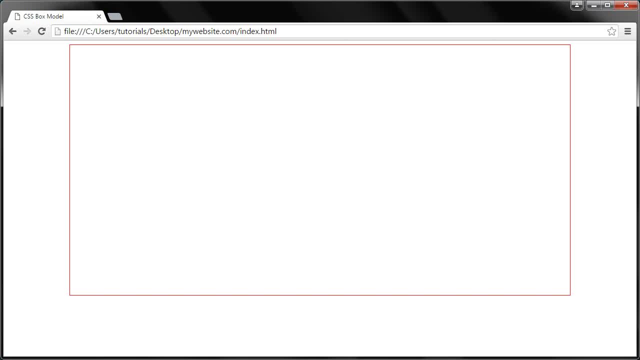 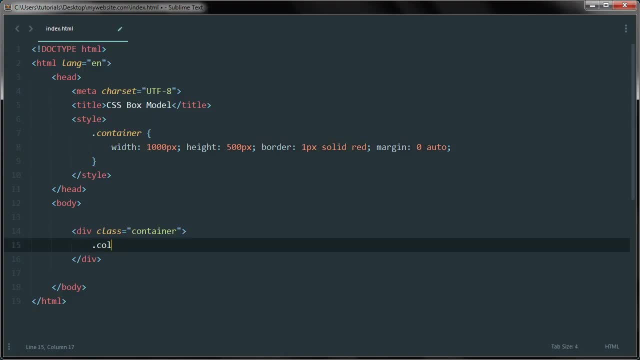 Thousand pixel container. Now, inside of this, I want a four column layout. So the way we do that is: inside of this container we have a column class and I'm just going to keep it like this for now. No, in fact, I will add some content, I'll just do a paragraph and I'll add some lorem. 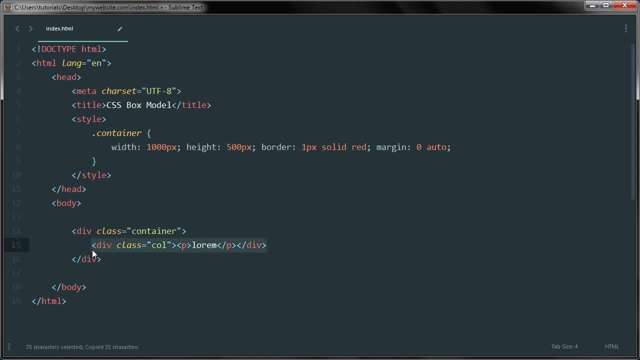 in there. So I've just put it on one line so it's easier for you to see. So if we duplicate this down, so now we've got our four columns. So now we've got our four columns And we need to target that with CSS, So we'll do coal and we'll set the width. 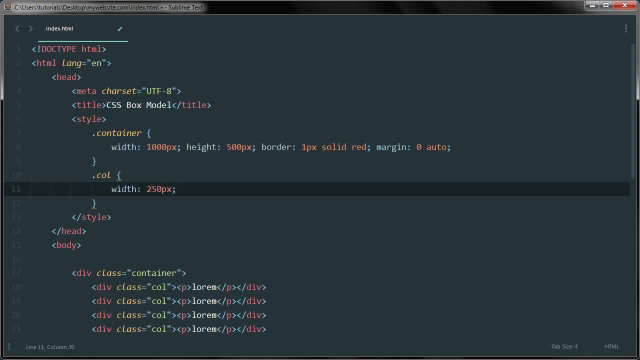 to 250 pixels, because four times 250 is 1000.. I'll just do a random height in here for now of 300 pixels And I will do a background color And I'll set that to yellow And then just to get. 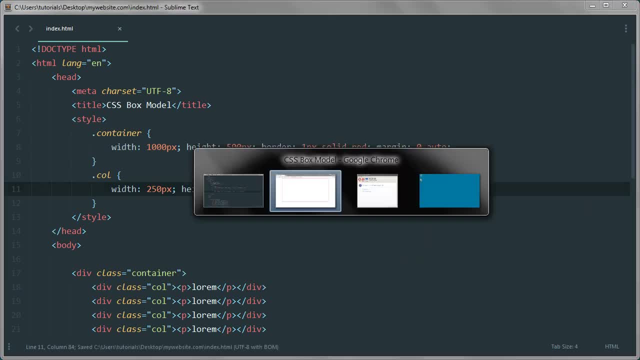 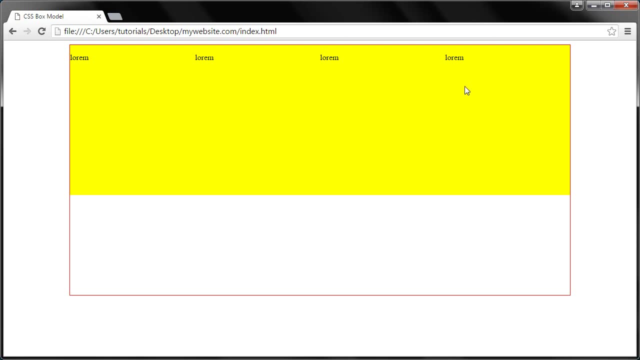 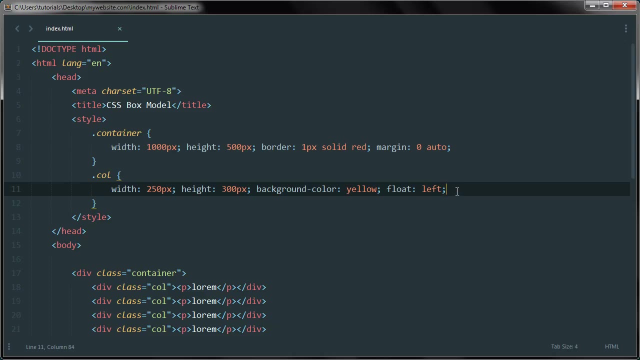 these all in line. I'll float those to the left. So now if we take a look, we can see that we have our four columns with the yellow background and because they're 250 pixels wide, they fill up the space perfectly. There's no white spaces in here. Now let's say we wanted to add a property onto. 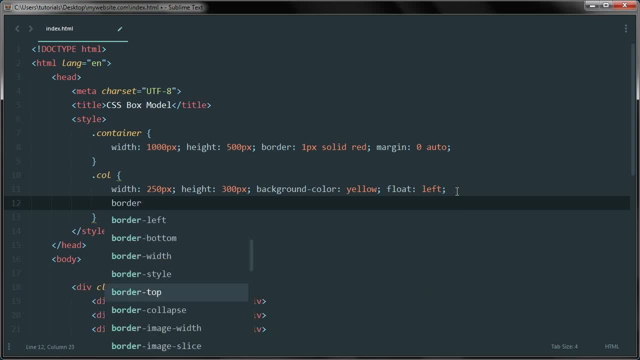 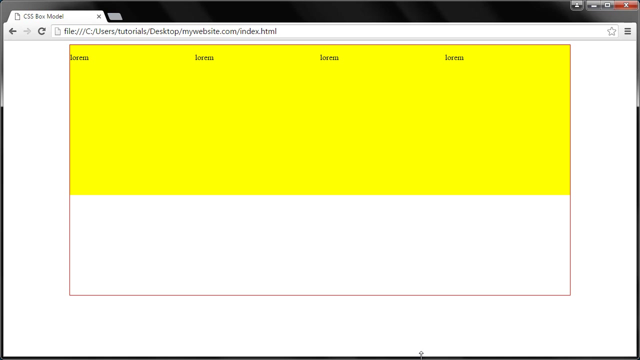 this Now let's just start by adding a border, And we'll add the border to all four of the columns and to all four sides, So we'll do one pixel solid And we'll do black. So now let's take a look at what happens to the result in the browser. So at the moment, 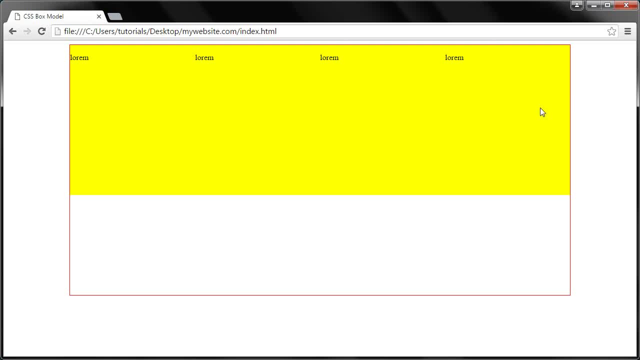 we've got 250 pixels. times four is 1000.. So it fits in the container. But when we refresh you'll see that the end column drops down a line, And that's because we've added a one pixel border here, and here times that by four, So that's eight extra pixels. So now the full width here is 1008. 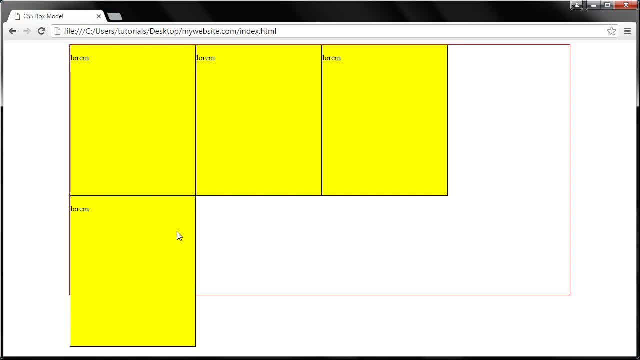 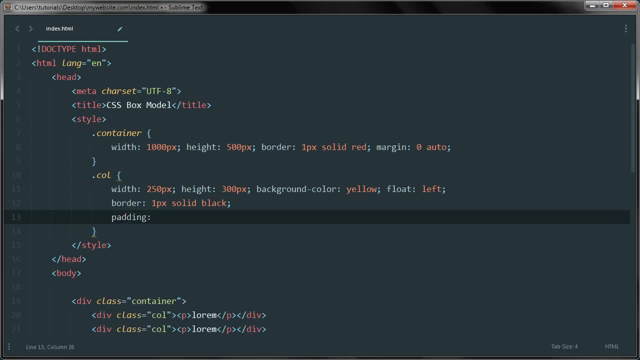 pixels, And that's just by adding a one pixel border. Now let's say I wanted to add a padding on that And let's just say I wanted to set that to 40 pixels And I also wanted a margin, So space between those columns. I wanted that just to be 10. 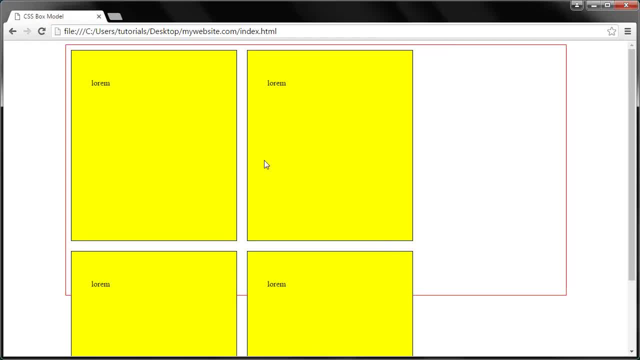 pixels. Now when we take a look, that really messes things up. So the box model has calculated or has rendered the actual size of the element by adding the width of the element with the padding, the border and the margin. So that's created the actual. 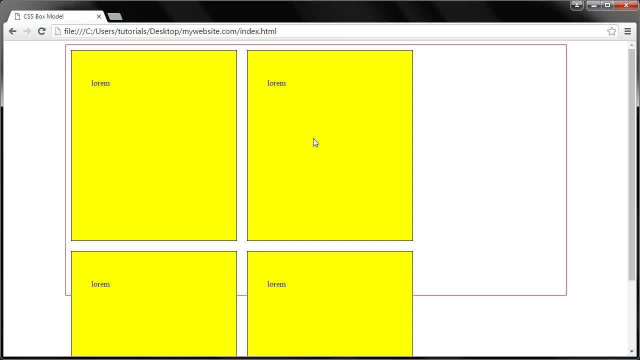 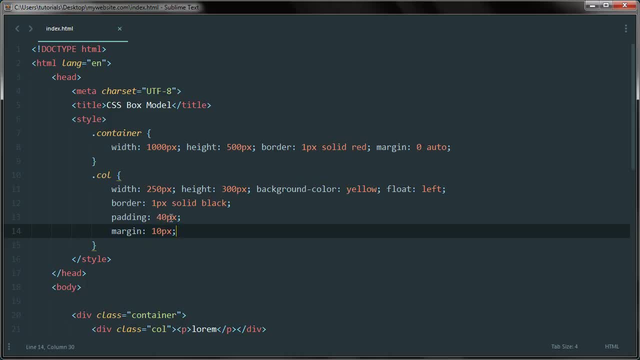 size of this. So if I wanted to get this working again, so that it's actually 250 pixels again, I need to take away 40 pixels from the left and the right, So that's 80. And then we've got our. 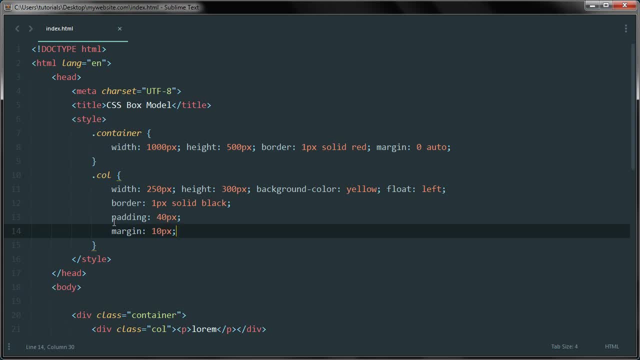 margin here, which is 20 on each side. So that's 100 in total there. So I need to take 100 off of this, And then I also need to take away two, because we've got a border on the left and right. 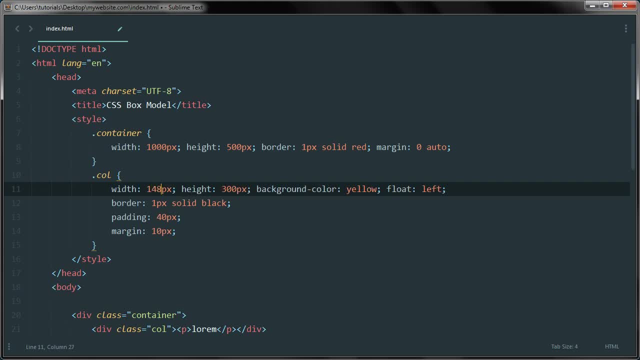 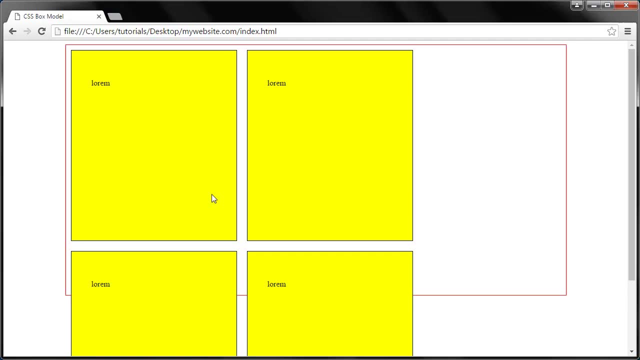 So that leaves us with a width of 148.. So 148 plus the 100 and the two is 250.. So now we've actually fixed this layout so that they are displaying properly. but, as you can understand, that is a real headache And to have to do that to. 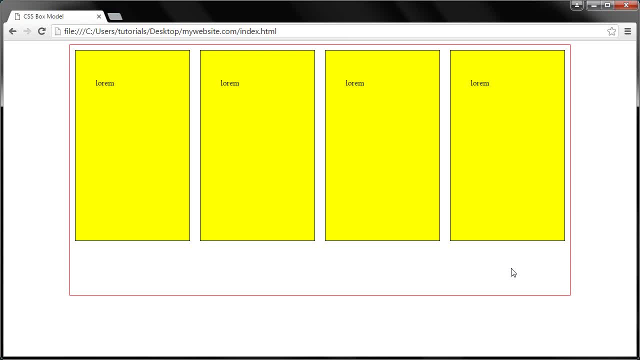 every element that you have can be a real nightmare. and even if you just change one value here- so let's say I want the pixel of the border to be two- that then affects the layout again and you have to go back and recalculate. so take another two off of here and you get the idea. so the